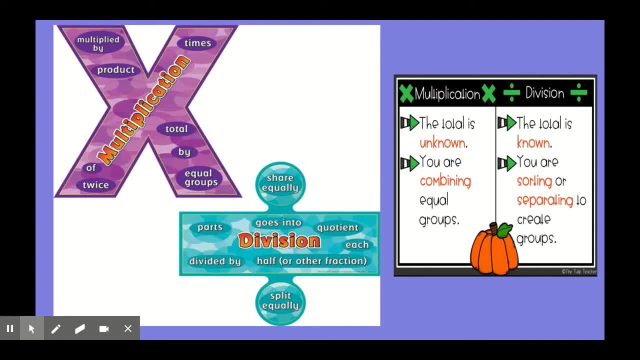 when to divide in a word problem, All right. so when we multiply, the total is unknown, just like in an addition problem. But in a multiplication problem you are combining equal groups. That is the key difference between when we add and when we divide. So when we multiply, the total is: 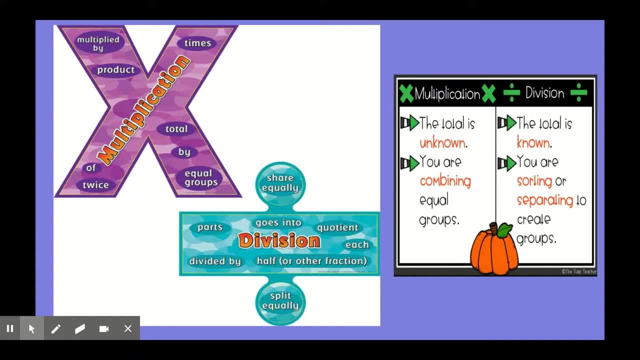 known. So when we add and multiply- all right, when you multiply, you are combining equal groups to find the product In division. the total is known. They will tell you exactly how many there are. It's your job in a division problem to sort or separate the total into equal groups. Okay. so when you're dividing, you are sorting or separating into equal groups. That is the difference between division and subtraction. So when you're dividing, you are sorting or separating into equal groups. That is the difference between division and subtraction. 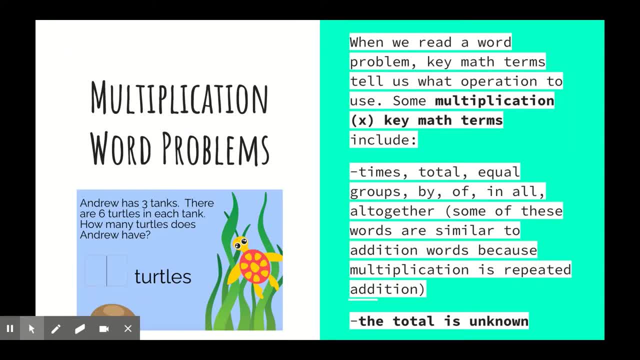 All right. so, as I said earlier, there's some key terms that tell us when to multiply, to use the x. These include times, total, equal groups by of, in all all together, And again the total is unknown. So, looking at this problem here, it says Andrew has three tanks. There are six turtles in each tank. How many turtles does Andrew have? 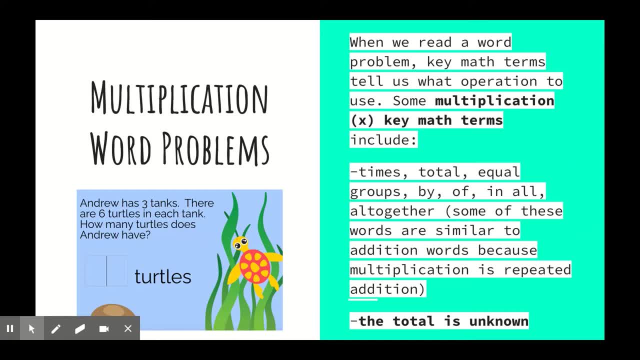 So I have three tanks. In each tank there are six turtles. How many turtles does Andrew have? So this involves groups, So I need to combine to find out the product. Okay, how many turtles there are in all. So if I have six turtles in each tank and there are three of them, I need to multiply three times six. My product is 18.. Andrew has 18 turtles in all. 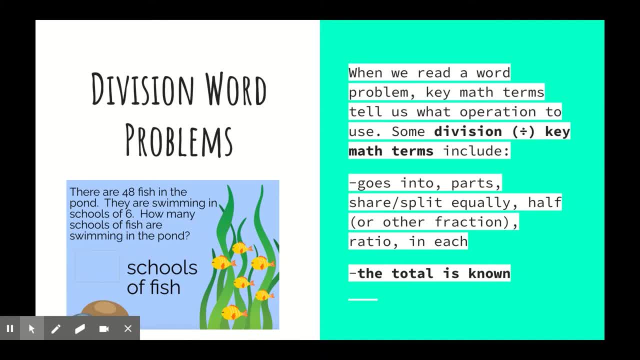 With division. as I said earlier, there are six turtles in each tank. How many turtles does Andrew have? All right? so, as I said earlier, there's some key math terms that tell us what operation to use to use a division operation. These also include: goes into parts, share equally, split equally half or other fraction word ratio. in each And again, the total is known in a division word problem. 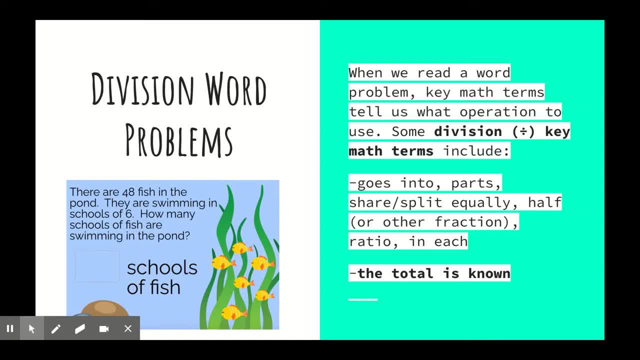 So let's take a look at the example here. There are 48 fish in the pond. That's my total. I know that there's 48 in all. They are swimming in schools of six. many schools of fish are swimming in the pond. So 48 fish and they are swimming in groups of six. 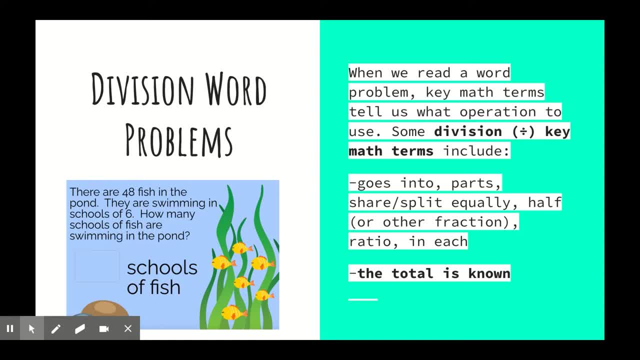 So they're asking me how many fish, or sorry, they're swimming in groups of six. They want to know how many schools there are, how many groups. okay, So we're going to divide. We're going to divide 48 by six to find out how many schools of fish are in the pond. okay, if they're each. 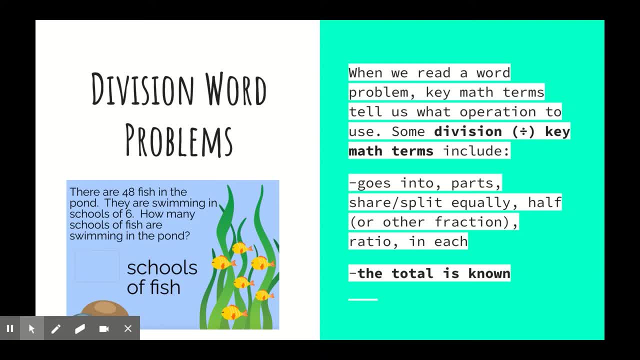 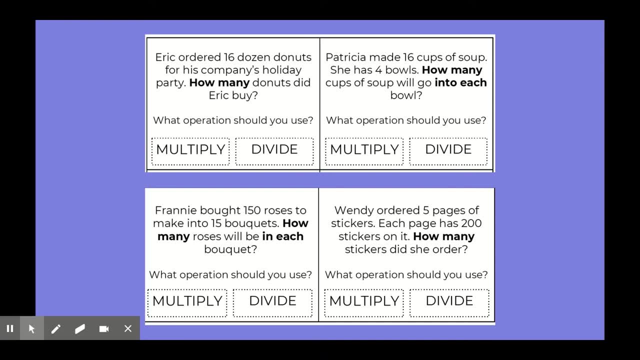 separated into groups of six. So 48 divided by six is eight. So how many schools of fish are in the pond? There are eight schools of fish. Let's look at some more examples of when to multiply and when to divide. The first example says Eric ordered 16 dozen donuts for his company's holiday. 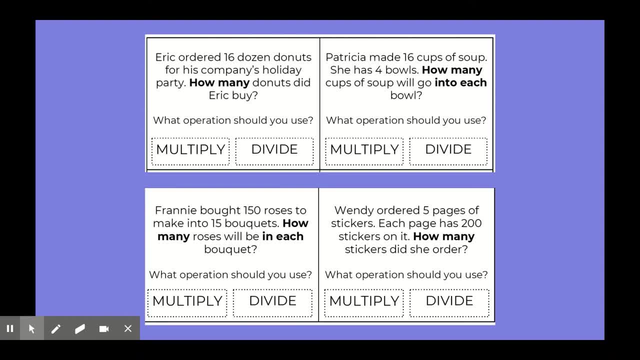 party. How many donuts did Eric buy? At first glance you might want to say Eric bought 16.. So for this problem you need to know some units of measurement. You need to know that a dozen is 12.. So if he ordered 16 groups of 12, 16 groups of 12 donuts, how many did he buy in all? 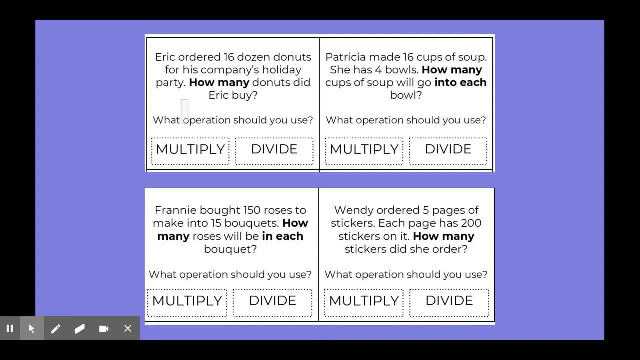 I don't know the total. so this is a multiplication problem. What am I going to multiply? I'm multiplying 16 times 12, and the product is 192.. Eric bought 192 donuts. The next one says: Patricia made 16 cups of soup. She has four bowls. How many cups of soup will go? 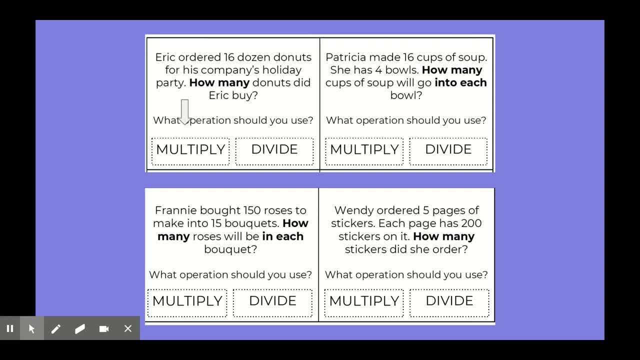 into each bowl. Well, I know the total: There's 16 cups. I need to separate it amongst four bowls or share equally. So my keyword here is: into each. I'm going to divide 16, divided by four, which of course is four. So each bowl will get. 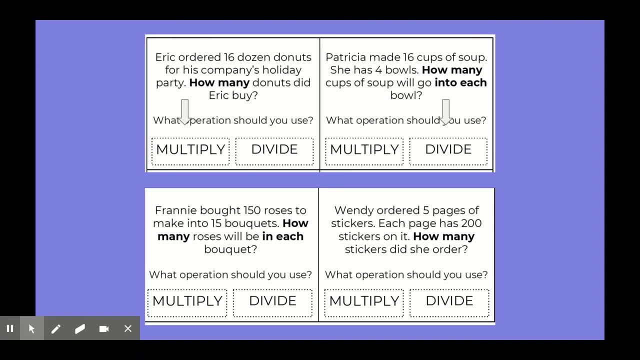 four cups of soup, All right, so that one's a nice, nice, easy problem. No remainders, They divide evenly. The next problem: Frankie bought 150 roses to make into 15 bouquets. How many roses will be in each bouquet? 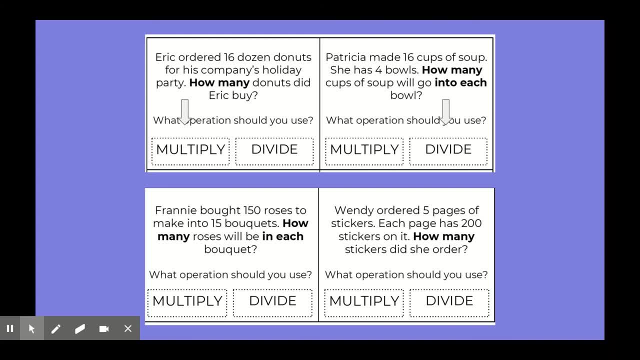 Again, I see the words in each. That means I need to be separating. I'm going to separate or divide. Okay, I know the total is 150.. I need to divide it evenly amongst 15 bouquets. How many roses are in each? There are 10 roses in each. We do 150 divided by 15.